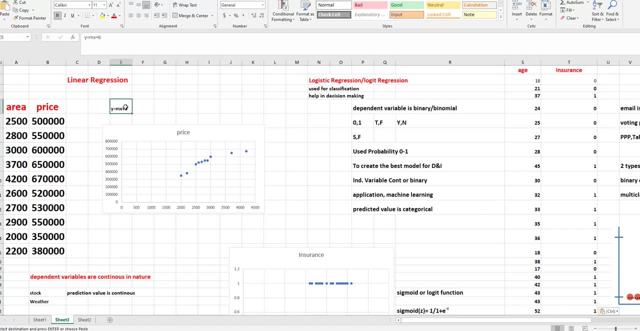 is intercept? if I is, if it, this is not clear. so I recommend please watch my video. I will also provide the link in my description as well. So the very simple. you can say that dependent variable in case of linear regression are continuous in nature, and here are the stock price, my example, weather price, these sorry weather. 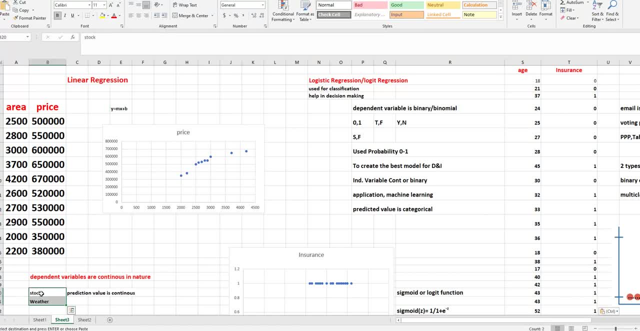 these dip. these are the dependent variable, means the stock price depends on the economy. So economy is the independent variable. and when we will make the model? so predictor value is continuous in the case of linear regression. Now we will talk about the logistic regression, which is also called. 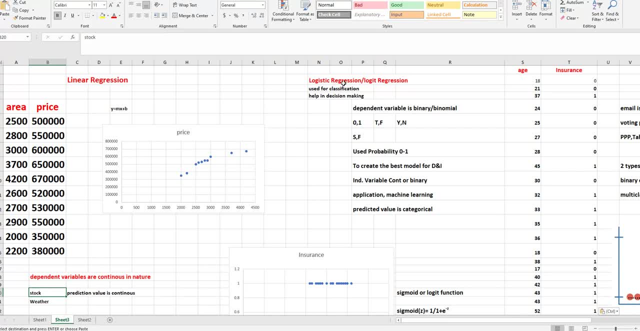 logit regression Do. the name says regression, but it is also called a classification. It works for as a classifier, so used for classification and it also helps in decision making. Now what is the meaning of use for classification? I have mentioned here there are two. 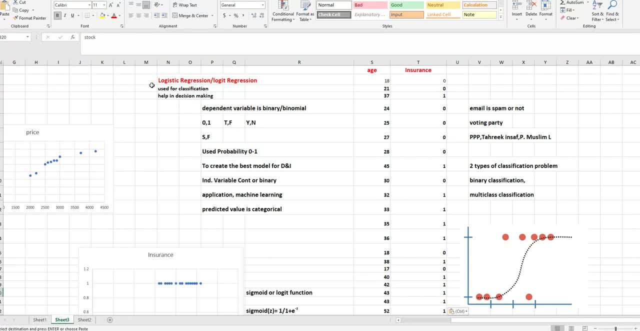 types of classification problems which we solve with the help of logistic regression. One is called the binary classification, which is our topic, and second is multi-class classification, which we will discuss later on. Right so, binary classification, or binomial means, which gives the output in the form of 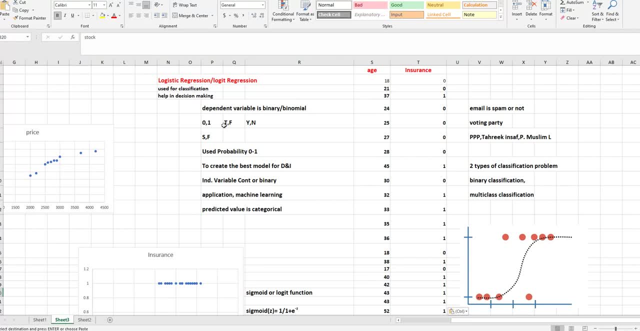 0 and 1.. Only there are two outputs: 0 and 1, true and false, yes and no, Right, success or failure. true means 1 and false means 0. Similarly, yes, y or s means 1 and f means 0. And it also helps in: 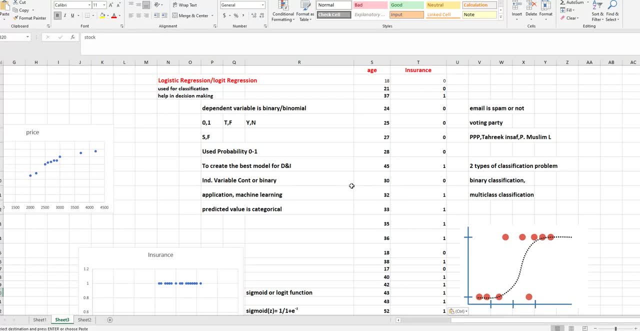 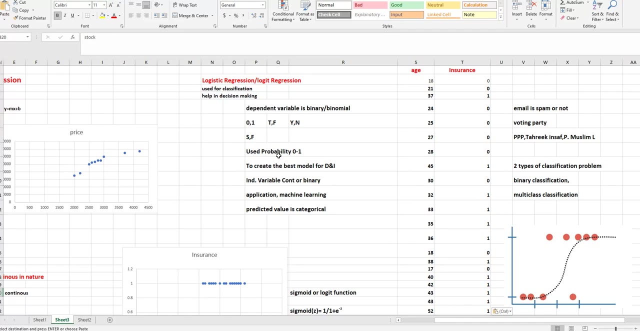 decision making Right when we have some problem in some situations. so we make decision by using the logistic regression Python. One of the most important feature is that the in logistic regression uses probability, and keep in mind that probability ranges between 0 to 1.. Whatever is the circumstances we have to create, 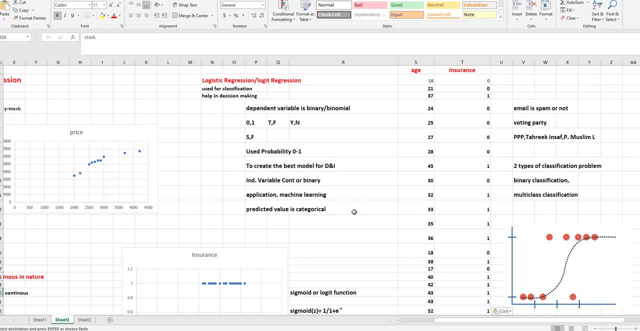 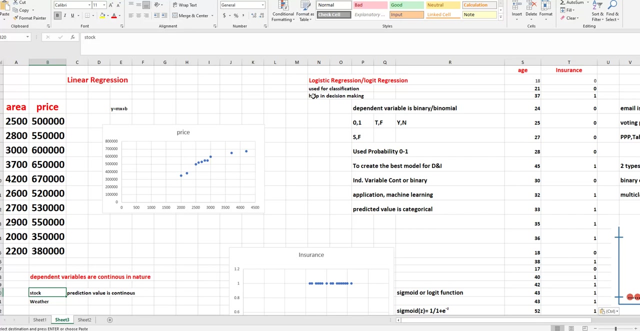 the best model for dependent and independent variable, while independent variable may be continuous or binary. Now the question arises where we use the logistic regression in machine regression learning. We use logistic regression in machine learning and predictive value is categorical. In case of linear regression, predictive value is continuous, while in logistic regression 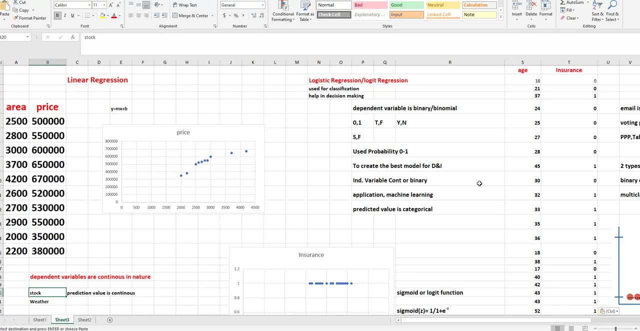 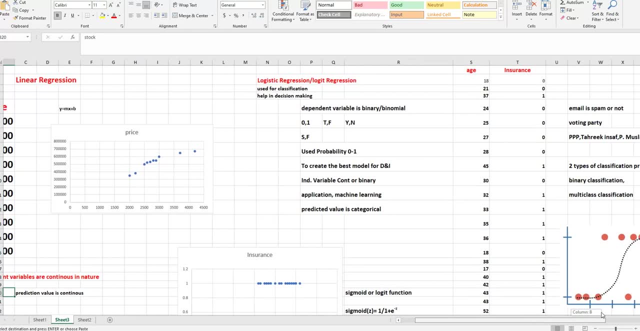 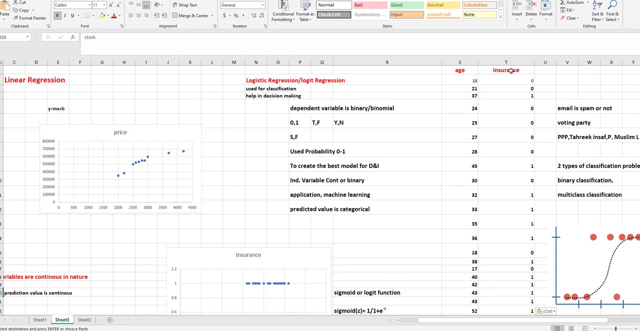 predicted value is categorical. Right? I will show all this with the help of example in my Python. This is just the background I am going to show and this example we will use in our Python coding. So see, here we have two columns: age and insurance. So if suppose the person is 18 years, 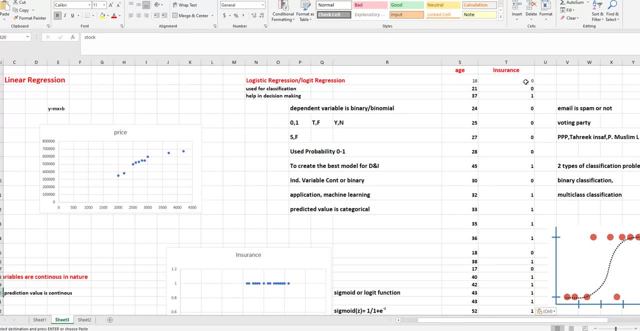 of her age. if I will ask him or her whether you want to buy a life insurance or not, maybe he will say no- 21 years. no 0 means no, 1 means yes If the age is 37 years. 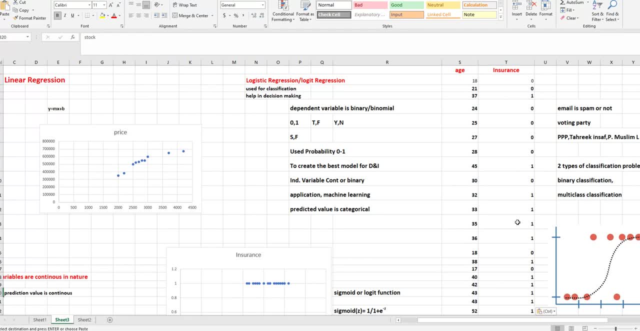 maybe he will say yes, so yes, Right. if you will see this pattern, you will see that the young people usually do not buy the insurance. as the age increases, the people buy the insurance. If I will make the graph by using these two columns, right, so I will get this type of graph. 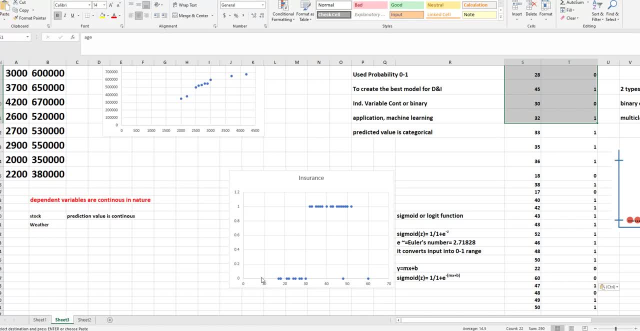 which I will show you here. See here: 0, as I told you that here we use in logistic regression, we use probability, and the range is between 0 to 1.. 0 means they do not buy insurance. but here is some outlier as well. Right, maybe at the age of 60 he does not want or she does not. 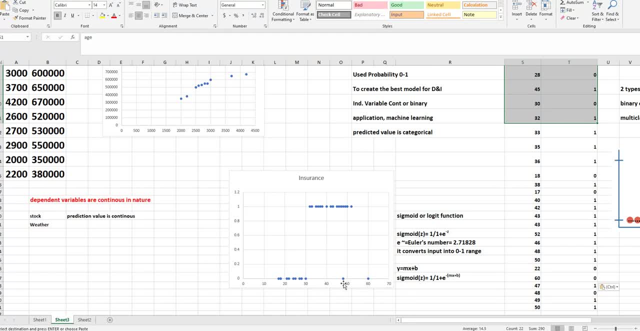 want 50. and here are: as the age increases. if you will see, as the age increases, people usually buy the life insurance. Now, if I will make the line here, hardly you can say one point will be on the line, So we cannot make any prediction, right? So in this case the graph is: if I will, 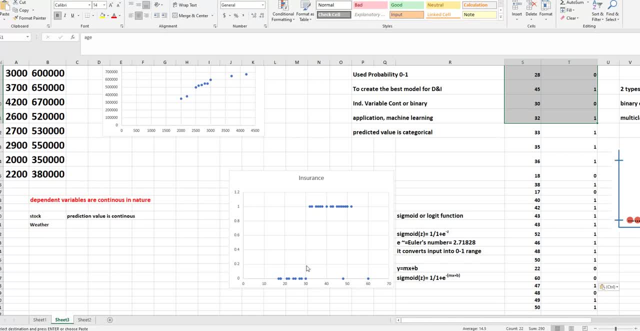 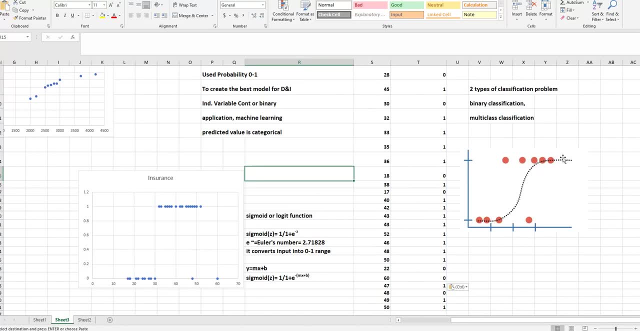 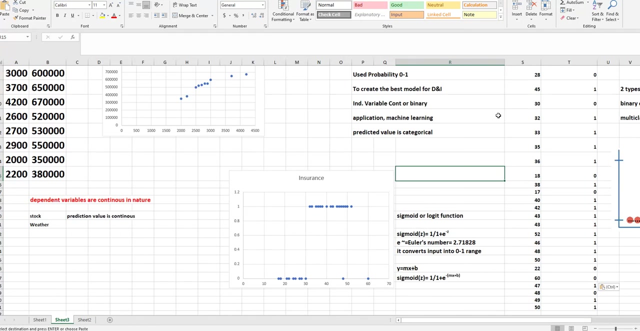 join all these points and then come down and join all these points, more or less, our graph will be just like this and s shape Right. it means these are outliers How we make this graph. so here is the term or the topic which we use in statistics, which is sigmoid function or logit function, If you. 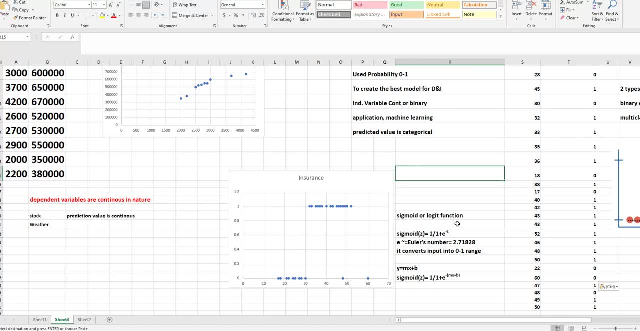 If you have a time you can read about the sigmoid function. but quickly I will explain to you that sigmoid. in some books you will see they have used letter P here. Some books they are going to use Z, but actually this is the probability, which is equal to 1 divided by 1 plus e, raised to power, minus z. 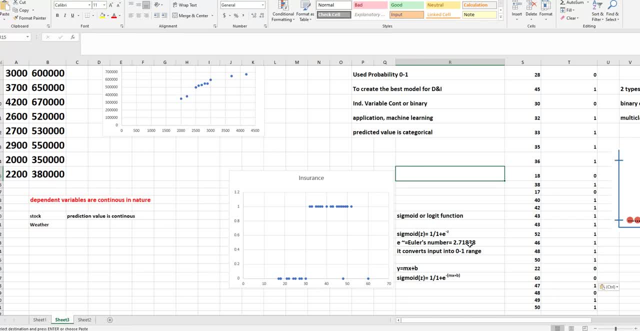 This e is called the Euler's number, which is equal to 2.71828.. What actually this formula sigmoid function does? It converts the input into 0 and 1, which is 0 to 1, which is the range of probability. But instead of this minus z, what you have to give here, you have to use this: y is equal to mx plus b, the value of this which we usually get by using the linear regression. 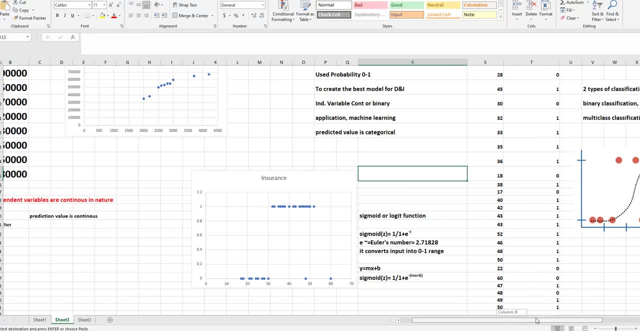 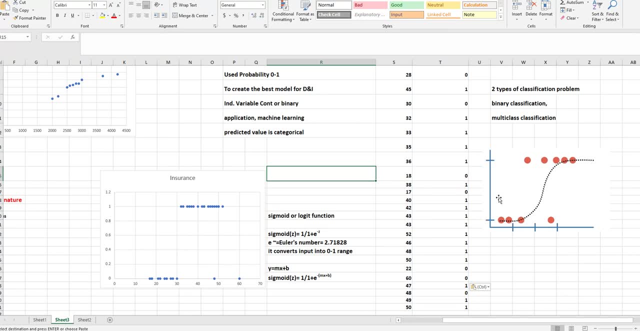 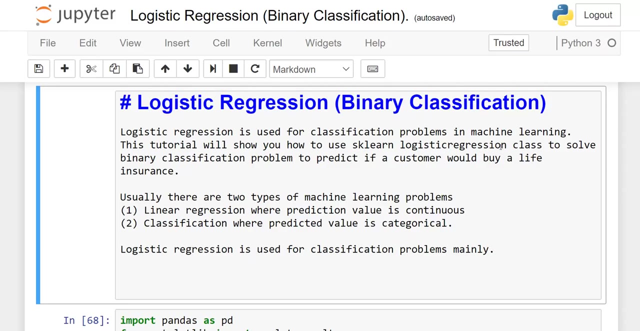 So this is all about this topic, which we are going to discuss when we will make the 2D graph. by using this sigmoid function, We will get this type of graph Right. OK, Now, we will, But this one. you do not have to worry about this, because everything will be so easy if we will do some coding in Python. 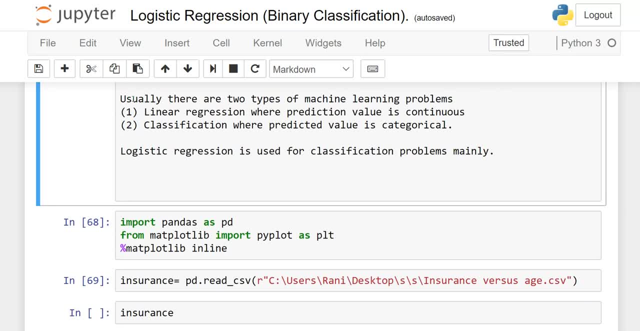 Right. So here I have written the same information that usually there are two types of machine learning problems: Linear regression, where prediction value is continuous, and classification means logistic regression, where predicted values categorical. Logistic Regression is used for classification problems mainly. Here we are going to discuss binary classification. 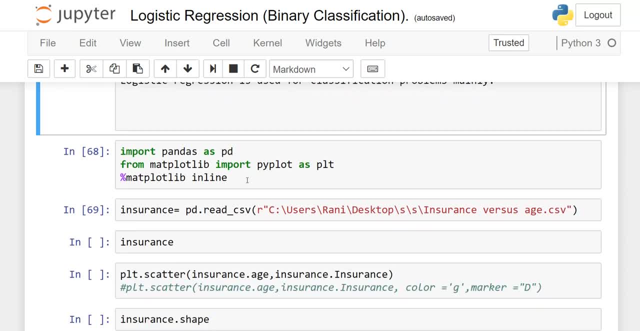 So first of all, you have to import pandas as pd, and you have to import matplotlib as well, because we will make some graph as well. When I will run it, you will see that it is executed successfully. Our next step is: we can wait. Asterisk means it's working. 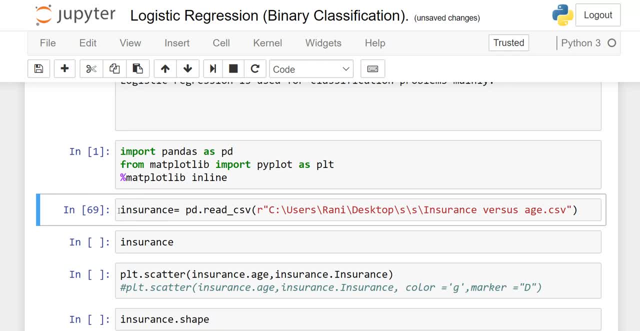 OK, So it's done now. So our next step is That we have to give some name to our data frame. I said insurance, right, because we are working on insurance and age, so whatever name you want you can give to your data frame, which is equal to pd dot. read and rescore CSV. now, with the help of read and rescore CSV, you can provide the path and quotation where your CSV file is located and executed. so see, it is executed successfully. 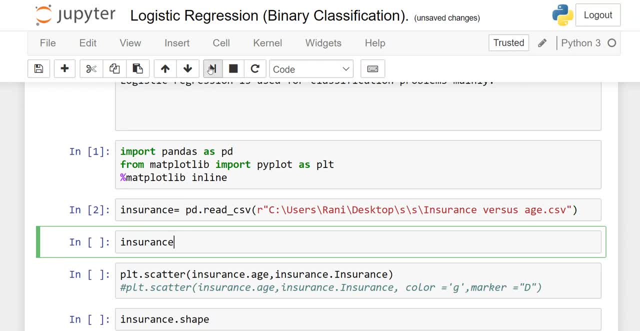 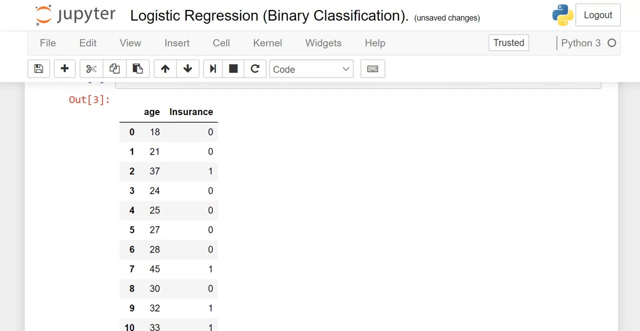 Now we want to check whether our data frame is here or not. Just write down the name of your data frame and execute it. it's here, exactly. you can see we have two columns: age and insurance. so randomly, if you will pick any number, you can see that 18 years 0 means he or she will not take insurance. 37, yes. 45, yes, right. 35, yes. it means as the age increases, people prefer to buy the insurance. 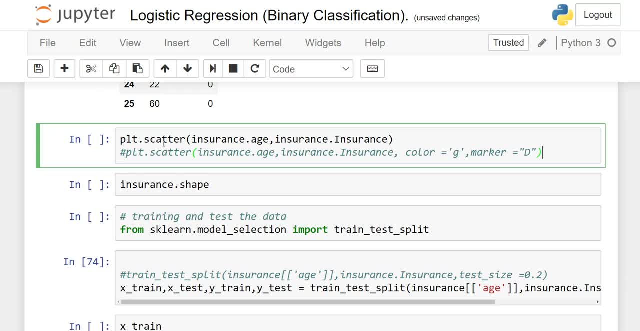 OK, Now if we will make some graph to show. So That is why we have imported matplotlib. we are going to make the graph between age and the insurance, plt dot scatter insurance. right, see, this is insurance name of our data frame dot. age. age is the independent variable and independent variable we take on the x axis insurance insurance, y2 insurance. this insurance is my data frame name and this, which starts with a capital, I, this insurance is my column right. 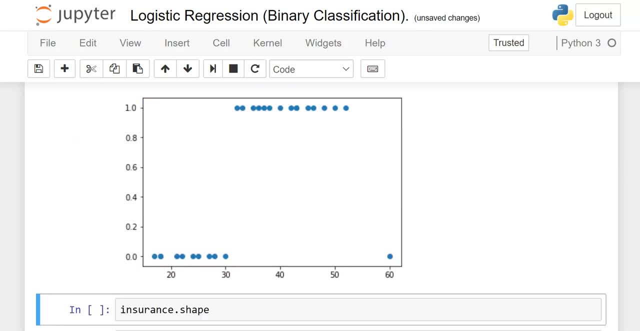 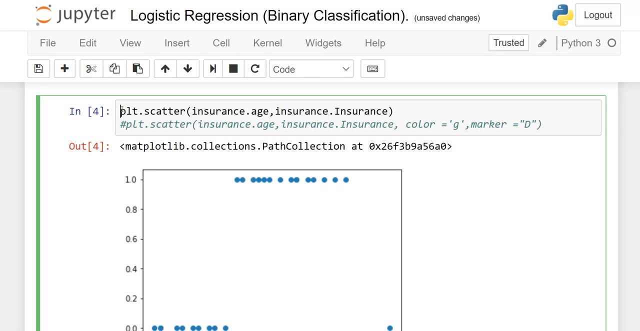 Run it So you will see that this is our graph. this is the outlier. when you will join this according to sigmoid function, you will get s shape curve right, and I had explained to you how it works. now I will make this comment and remove this hashtag. so color is equal to green. it is not necessary that you can write down this syntax. only if you want you can add some color. you can add some marker. I said marker is. 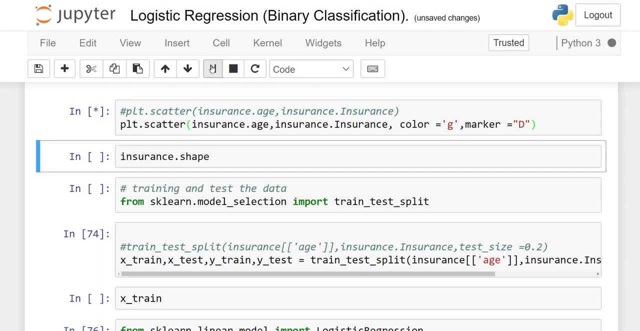 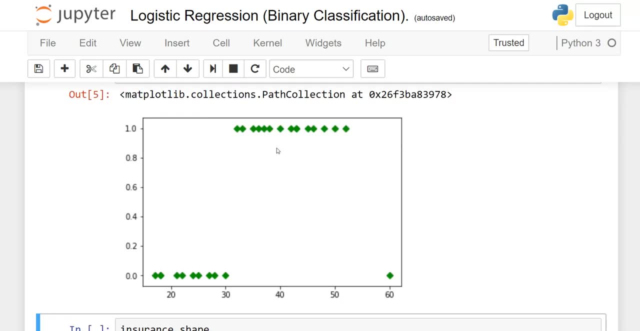 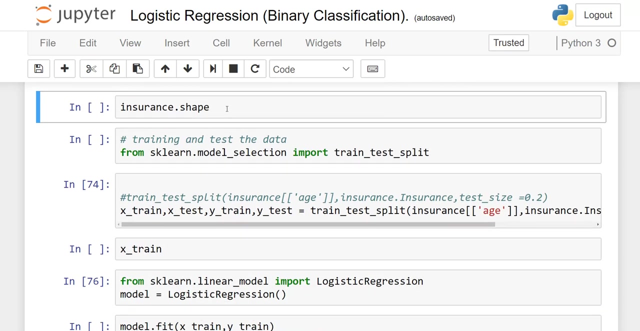 D means diamond color is green- and then run it. so now you will see this: the same graph, but now instead of circle we have by default it's circle. but if you want, you can change your marker as well. but if you will join again, you will see s type curve, 2d curve. this is the outlier. now you can play with it, make different colors, different markers. if you want to check the shape, shape means it will show you number of rows and number of columns of your data set. 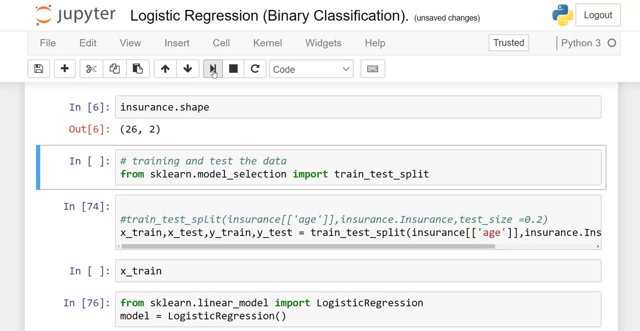 So. So, insurance, name of your data frame, dot shape and execute it. it means we have twenty six records, twenty six rows and two columns. yes, we have two columns: age and insurance. it's all done. now we are going to split our data frame, which is which is consists of twenty six records. so training and test the data again. this, this topic we had discussed in our last lesson as well. you have to. 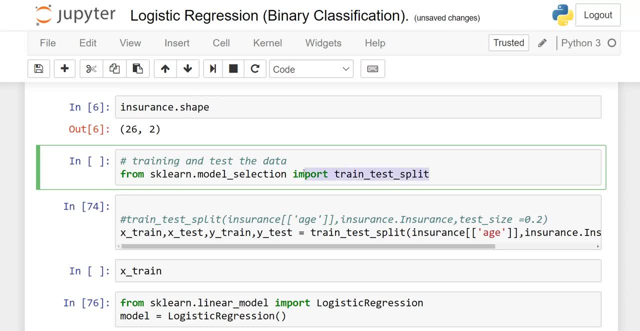 Import Train underscore- test underscore is split from SK. learn now what will happen. we will split about twenty six records, maybe fifty, fifty percent, it's up to you- eighty percent or twenty percent, seventy percent or thirty percent. so here I am going to split between eighty and twenty percent. twenty percent as a test and eighty percent as a training. I am going to train my data and for twenty percent I will test my data. 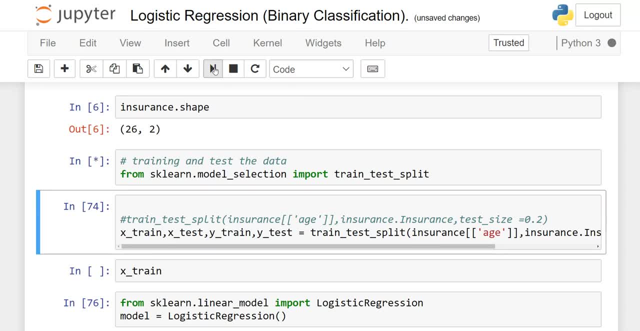 Now how to do after this. I will execute it. it's executed. see as trick when it's working. so we will. okay, we will discuss this. it's done. now See this one. the right hand side of this is exactly same what I have put a comment here, only to show you how you have to write down train underscore. test underscore is split. this one because we are going to split our data. this is my data frame name. this is the syntax. 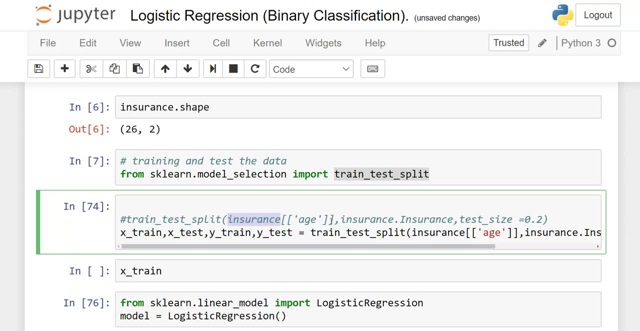 Age: right, you have to write down independent variable in two DRA. two DRA means you have to use two square bracket. insurance dot. insurance test size is point two. point two means twenty percent. whatever is the twenty percent of twenty six records, we will apply testing and eighty percent is our train model right. so exactly from here to here. I have written in my second line. you can see here, but what output we will get, that is. 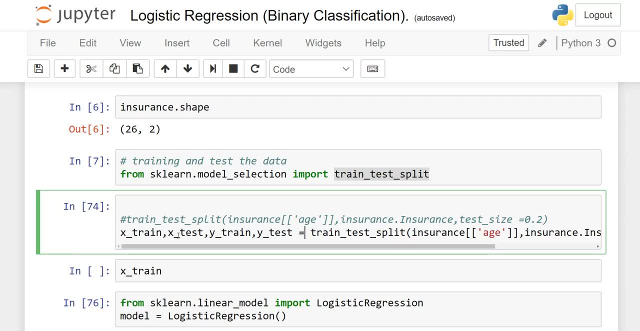 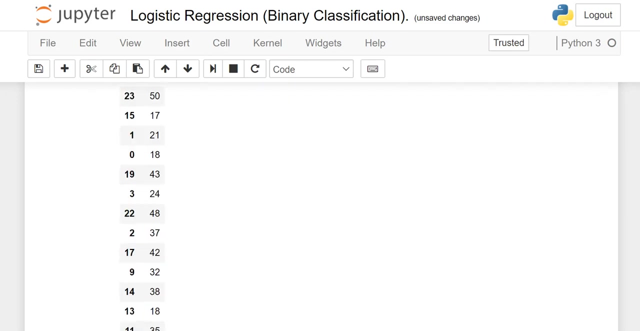 I have made two lines equal to X train comma, X test, Y train and Y test. so first of all we will check X underscore train. right, I will execute this first, otherwise it will not work. okay, X underscore train. so whatever is the eighty percent of twenty six records you will see here. so see if you will count. these are not twenty six, this is the eighty percent. but 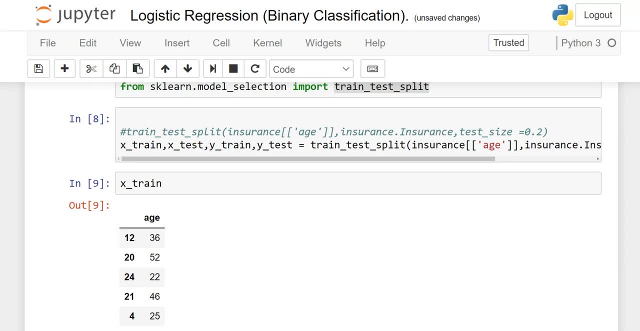 It will not give the output of first eighty percent or the bottom eighty percent randomly. it will pick eighty percent. so first he paid the stories, the first, the system pick twelfth record, which is thirty six, and then twenty record, twenty four and so on. similarly, if you want to check for why, just make it? why it will give you the output eighty percent randomly records eighty percent. twelve record one. one means he or she will buy one. 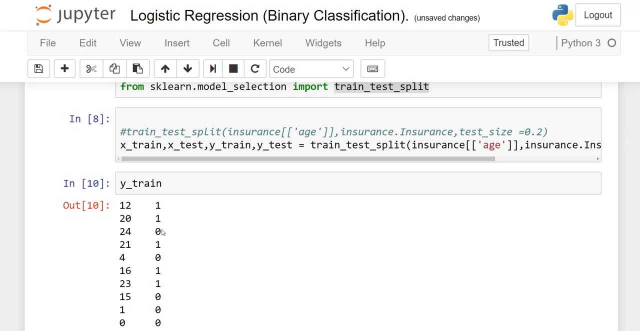 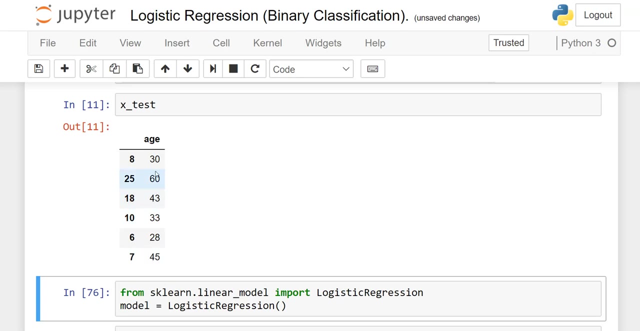 the insurance 24th record: she or she will not buy the insurance, right? okay, now for the test. for the test is whatever is 20 of the 26. so these are one, two, three, only six records, 20 of 26, which so 8, 20 feet, again randomly, it will pick, right, i am going to make it train here again. 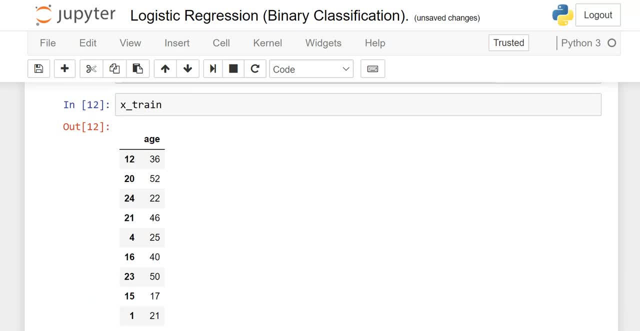 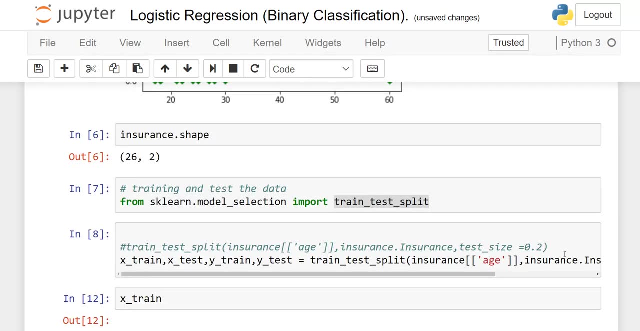 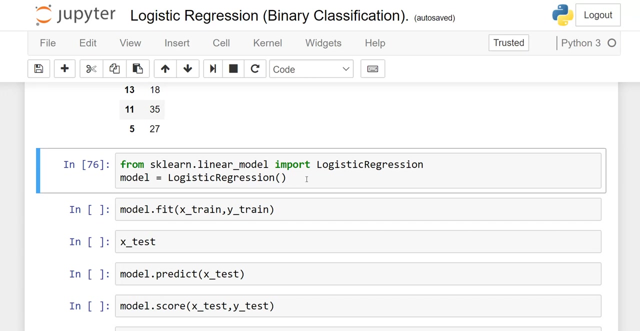 because we will use test later on, right? so train is 80 percent, test is 20 percent. it's not necessary that you have to keep this ratio. 30 percent, 70 percent is up to you now. here, when we made our split. here, we have to import logistic regression and we have to create our object. so from sk, learn. 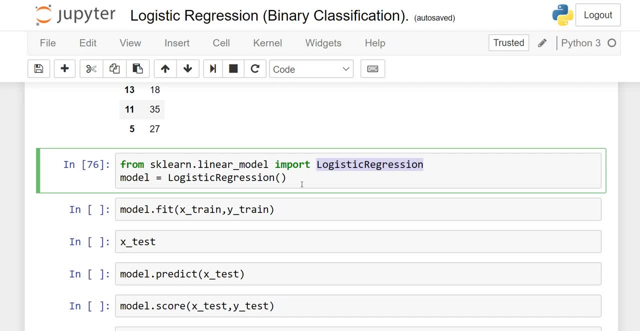 you have to import logistic regression and from this logistic regression we have to make our model object. sorry. so, whatever name you will use here, same name we have to use in rest of our coding. so model is equal to logistic regression. and then parenthesis, and then i'm going to run it. it is. 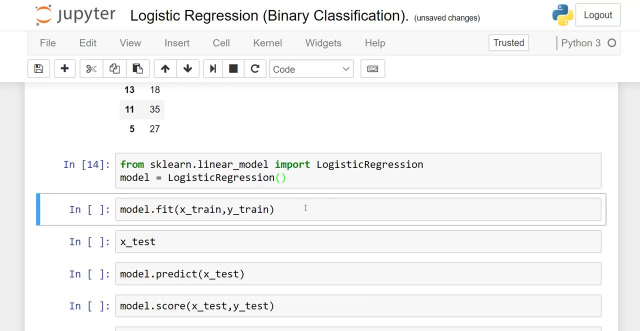 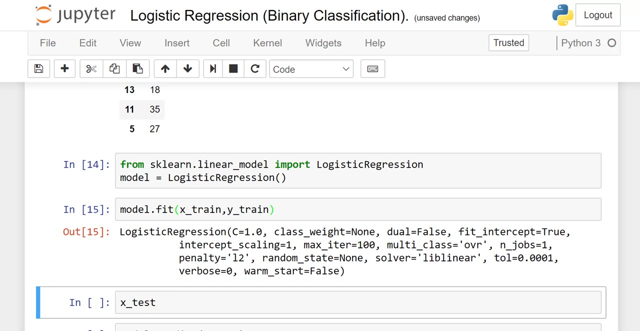 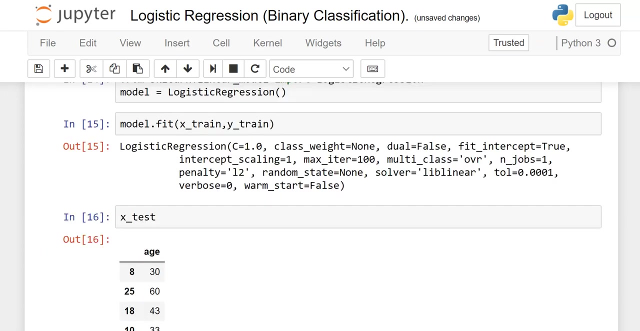 successfully executed. now our we have to fit our model. here means dot fit function means that we are going to make our model and see it is successfully created. now our test again: x test, which is the 20 percent of our record. so here is the 20 percent. 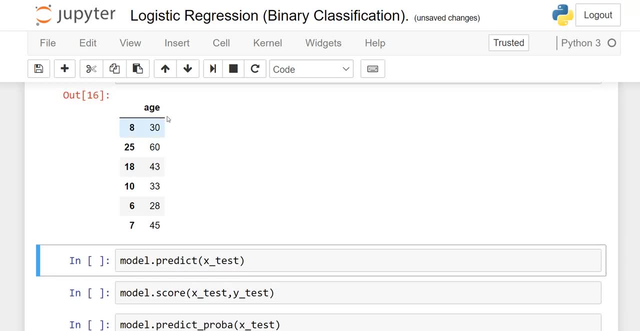 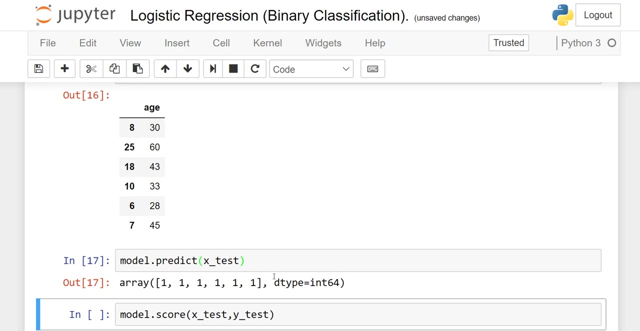 of our record. the system picked eighth record, 25th, 18, 10, 6 and 7. now we are going to predict model dot, predict x, test right, what is the output? i will show you. then we will discuss. so see, one one one. what is the meaning of this? one one one means the first record is 30 years. he or she. 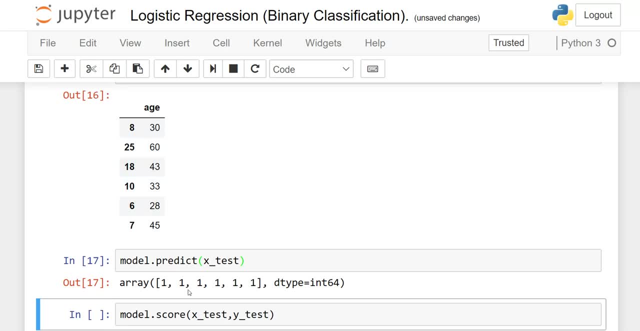 will buy the insurance. yes, one means yes, 60 years, yes, 43, yes means all will buy the insurance. one, one, one, one one means we have seen in our scsv file that as the age increases- starting from 17, 18, 19, 20- they will not buy the insurance. but see these as the age increases they. 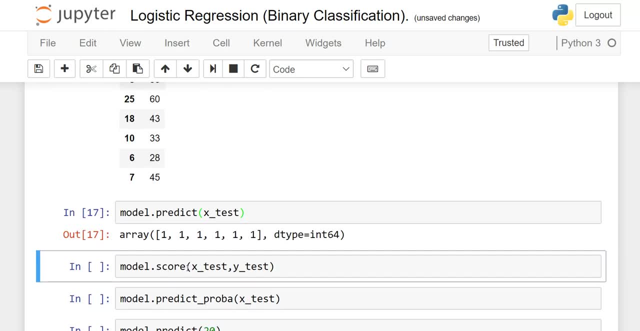 will buy the insurance. so if you want to check the score, a score means it will check what is the relationship, how perfect your model is. when i will run it it says 0.5. it means our model is 50 percent accurate. right is not one. one means every, each and every figure is correct, but it is. 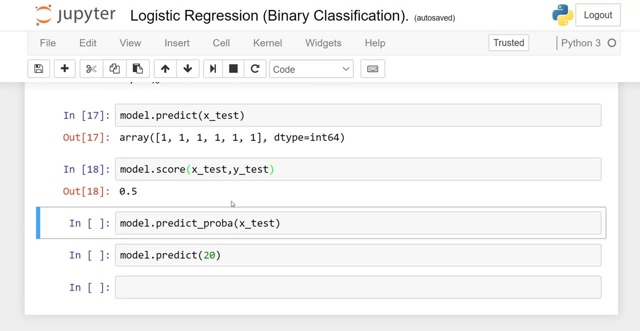 50, 50 percent. so dot score. with the help of dot score you will find out what is the relationship between these two variables. so more model: dot predict in probability. in case of probability, you have to write down dot predict underscore probability. do not write down the complete word. 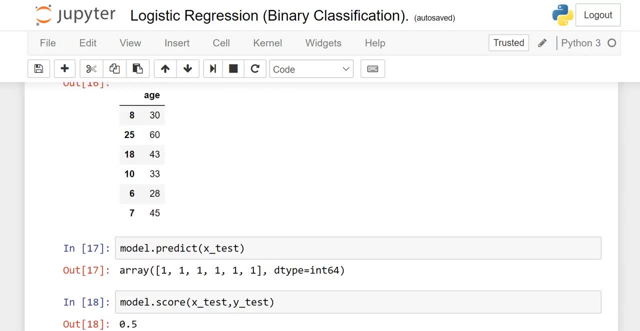 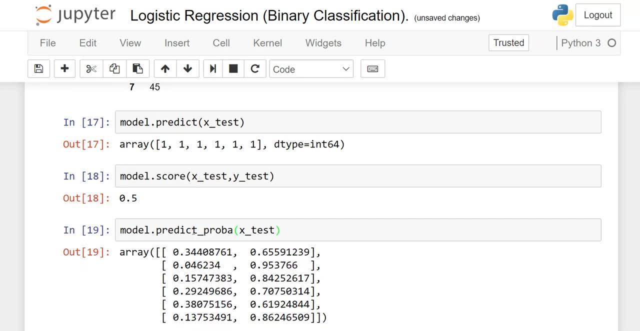 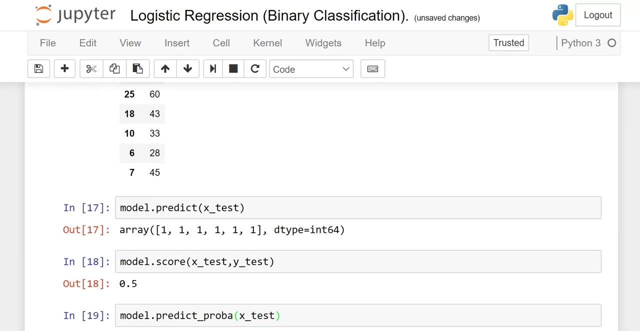 probability x test. right, we are going to see these. these are the test values. okay, first i will run, then i will show you what is the output. this is the output. see first one. if the person is 30 years, what is the probability first one will show they will not buy the insurance. 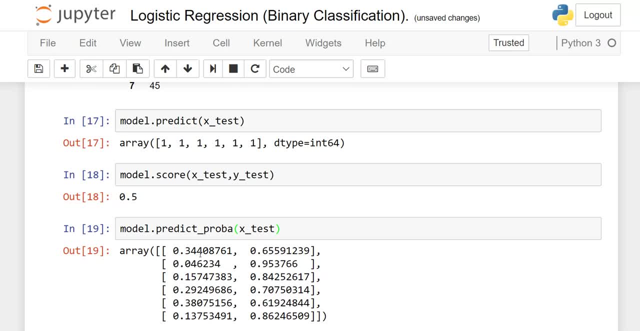 so point three. four means thirty-four percent is chances that that person is not by the insurance. 65 percent is probability that he or she will buy the insurance. check for this last one: 45. see the age increases the chances of buying the insurance is more so. 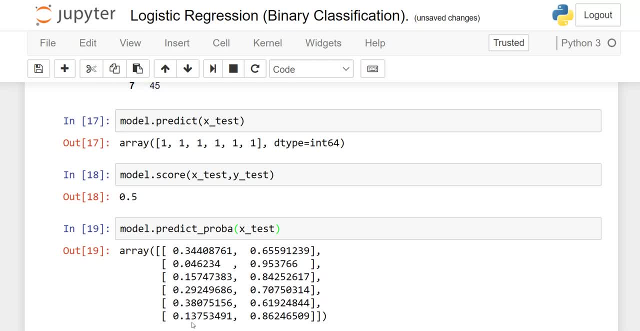 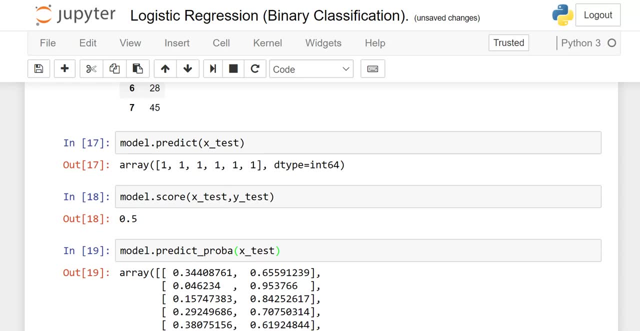 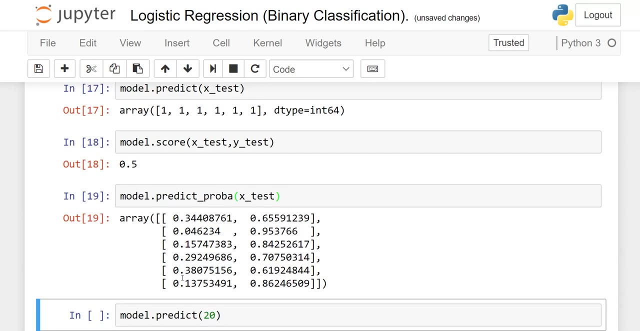 45 years means 13 percent probability that he will not buy the insurance, but there is 86 percent probability that he or she will buy the insurance. take one more example. right, this is 28. we will check the second last. so what is the second last? 38 percent probability that he or she will not buy. 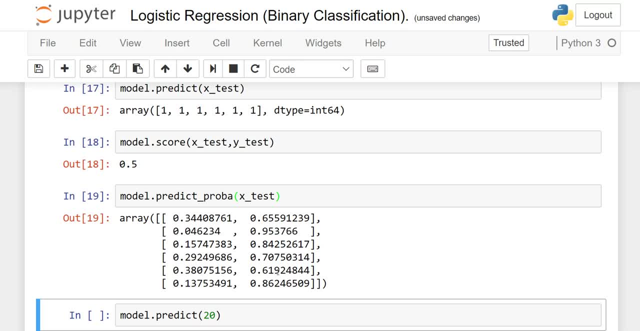 the insurance, but 61 percent probability that he or she will buy the insurance. so if you want, you can check dot predict underscore probability. the first one will show not, not, and this will yes. so no and yes probability right here. if you want, you can use some age. 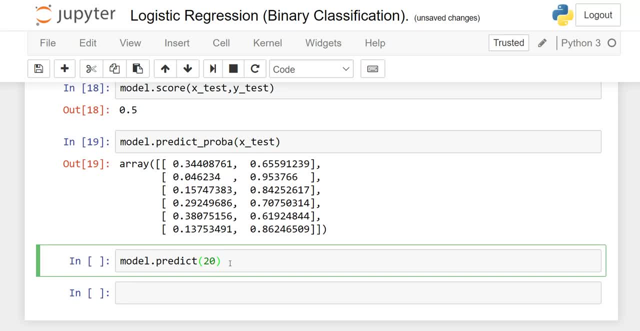 dot predict parenthesis. we can write down 20 years. if the person is 20 years, he will buy or not? so answer is no, because young, our data says as the age is less, he or she will not buy the insurance. i am going to make it 70 and when i will run it? so it is one. one means yes, he or she will buy if i will. 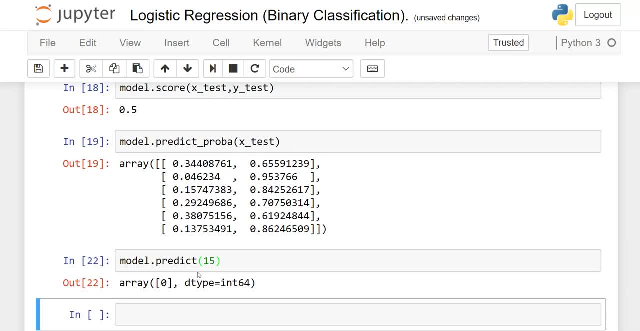 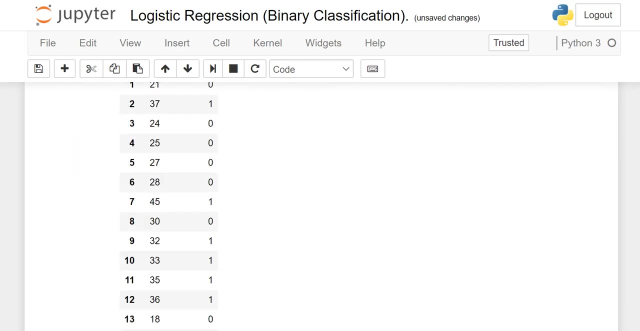 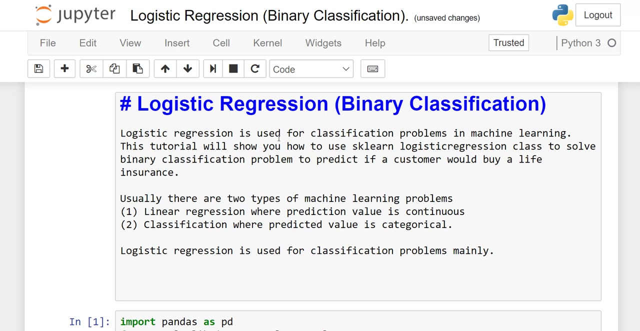 make it 15, which is young again, the output should be zero. if i will make it 45, it should be one, and which is one. so see, here, with the help of this model, we can check our test as well. so i hope that this is this topic, logistic regression- which is one of the most important topic in machine. 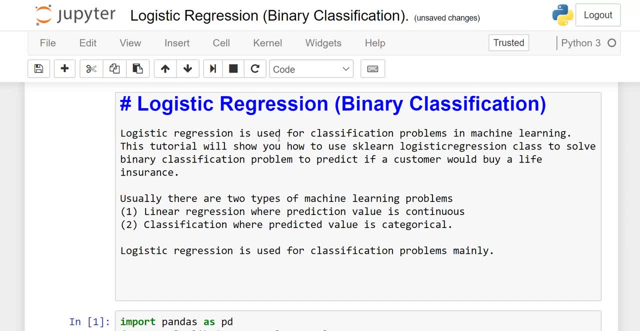 learning is clear, so please practice it. see you in the next lesson and thank you.